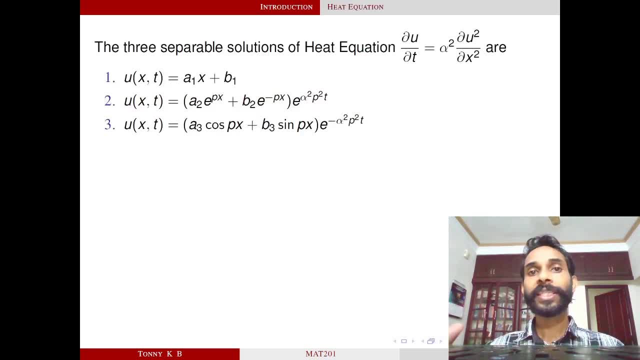 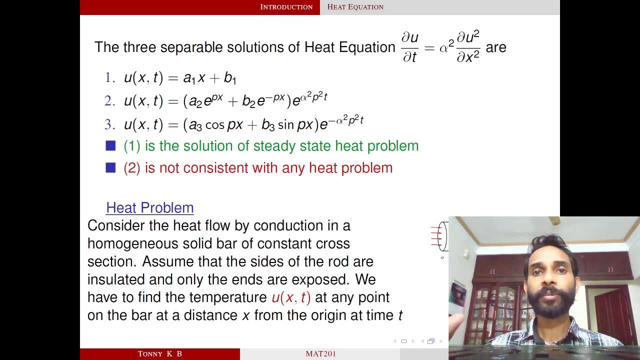 Namaskaram. in previous session we have derived three separable solutions of heat equation. Also we have seen that first one is the solution of steady state problem and second one is not consistent with any heat problem. In this session we will derive Fourier series solution. 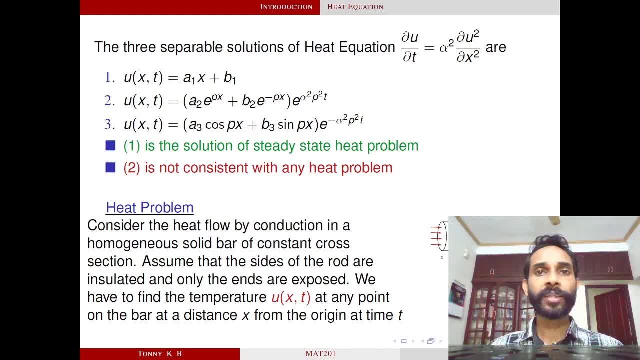 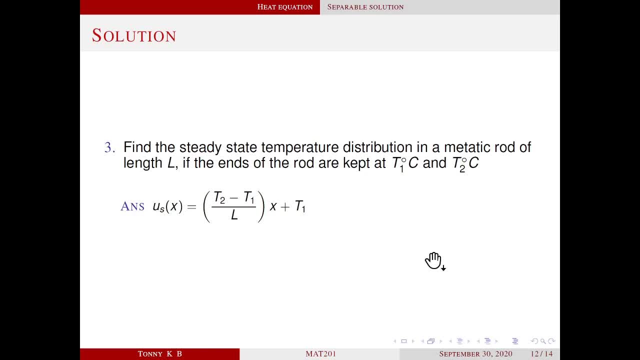 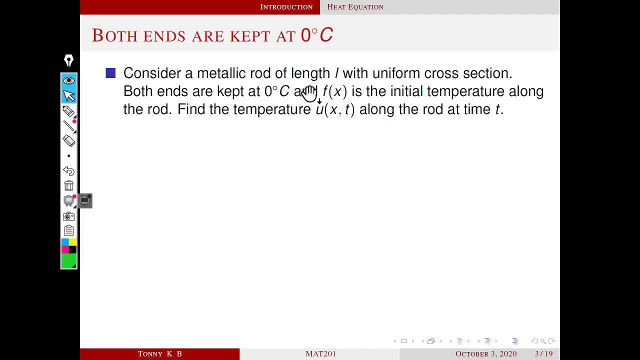 of heat problem with some special boundary conditions. Ok, let's start. This is the solution of previous homework. This is one of the special case. Both ends are kept at zero degree Celsius. We consider a metallic rod of length L with uniform cross. 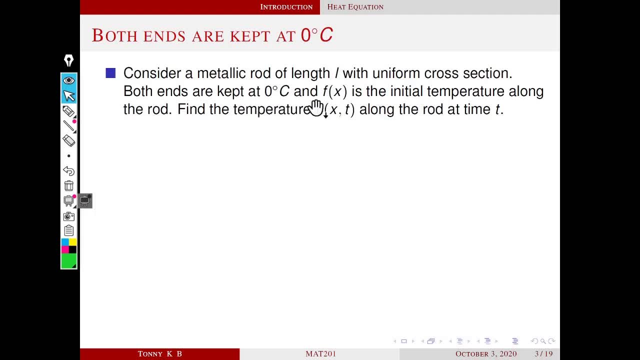 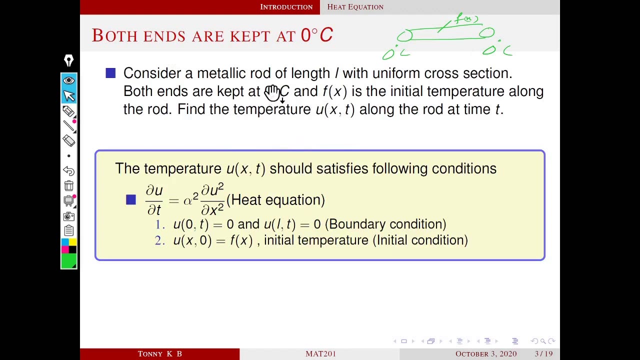 section, And here both ends are kept at zero degree Celsius. And what is f of x? f of x is the initial temperature distribution And we have to find u, X, t. Ok, And this is is the mathematical version of this problem, because we know that our temperature function. 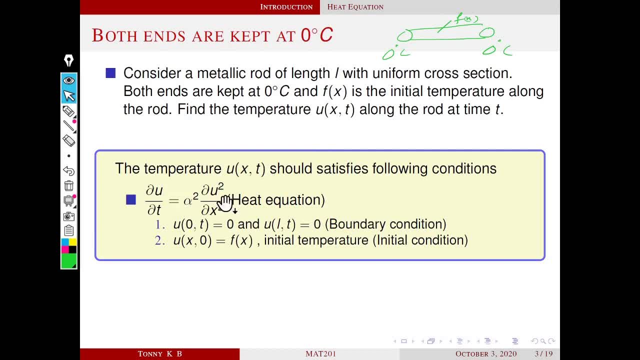 uxt satisfies heat equation, So u should satisfy this equation. and also it is given that u0t, that is temperature at x, equal to 0. that is descent, that is always 0, and similarly temperature at descent. the length of the string is l, so that is ul t equal to 0, and next one initial temperature. 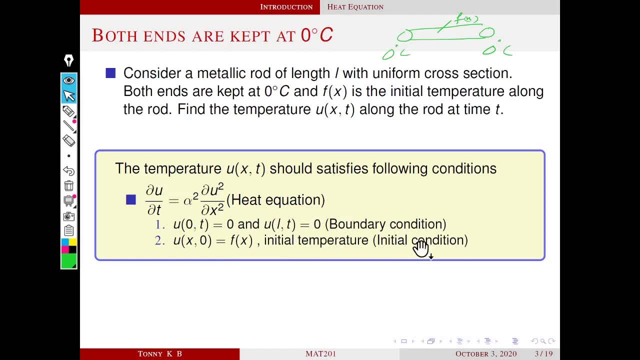 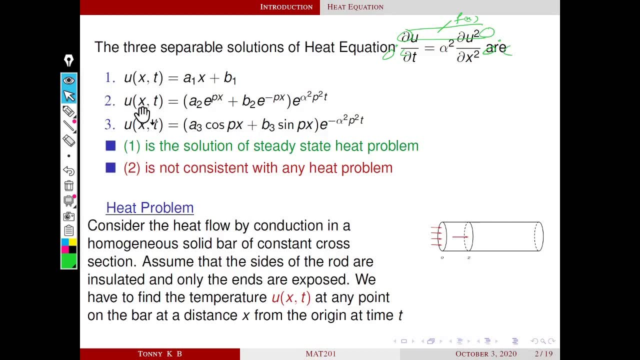 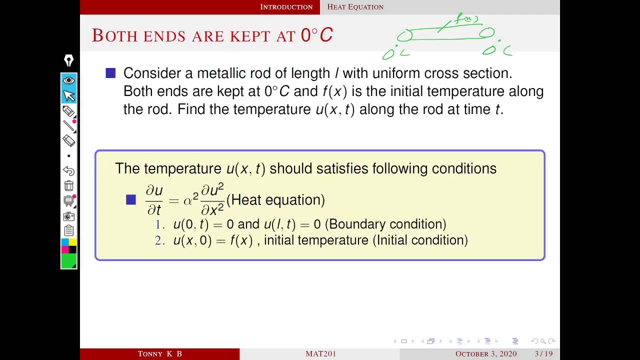 when t equal to 0, our temperature is f of x. this is the initial condition. these are the boundary conditions. Already we know that first one is the solution of steady state problem and second one is inconsistent with any heat problem. So let's try this problem with the third solution, that is. 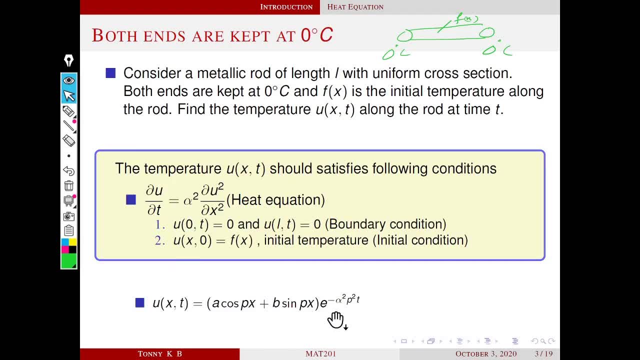 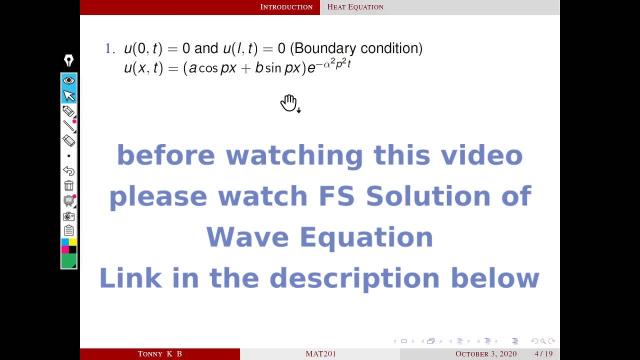 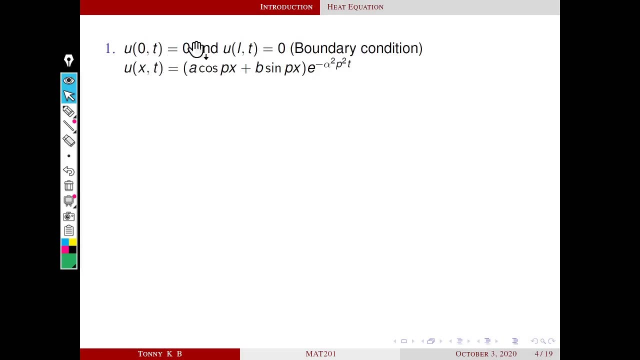 uxt equal to a cos px plus b, sin px into t raised to minus: alpha square p square t. The derivation of this solution is almost similar to Fourier series solution of wave equation. First we are going to apply the boundary condition on the solution uxt. So first we apply the condition u0t equal to 0, that means when x equal to 0. 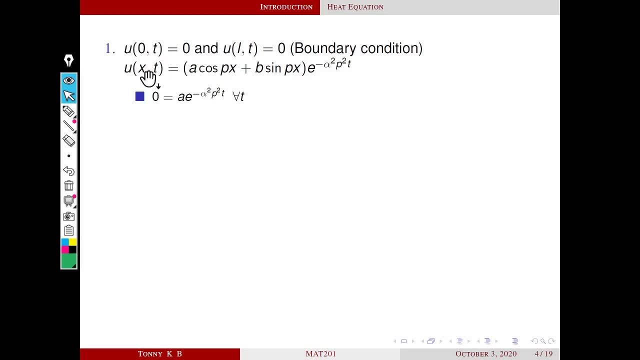 temperature becomes 0, substitute x equal to 0, so left side becomes 0 and right side is here. cos 0 is 1 and sin 0 is 0, so a into raised to minus alpha, square p, square t, for all t, and we know that this. 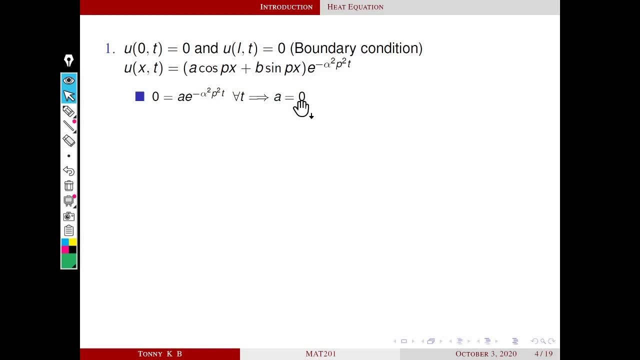 is true for every equation. So let's try this problem. So let's try this problem. So let's here this areaMy equation is going to be 0, this areaO is equal to 0 and this is going to be t. how did be? would you substitute t only when a equal to 0. okay, so you simply substitute a. 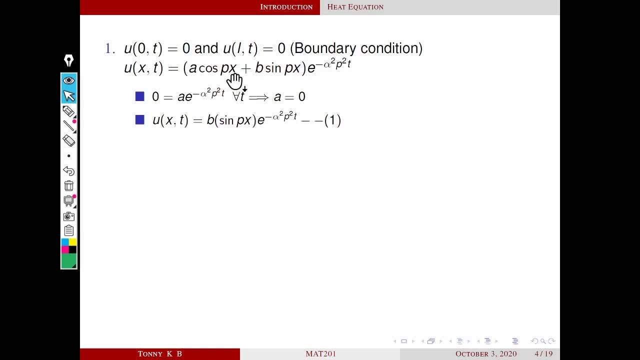 0 in. this is the solution. so what happen? so our uxt become b, sin px into e raised to minus alpha square, p square t. we denote this equation by 1. next we apply the second boundary condition, that is, substitute x equal to l. when x equal to l, left side become zeroan right hand side become b into sin p, l e raised to minus alpha square, p square t. this is true for every equation only if we notifications I'm going to use two boundary conditions. so hereそして haciendo unaử hahba basccal. 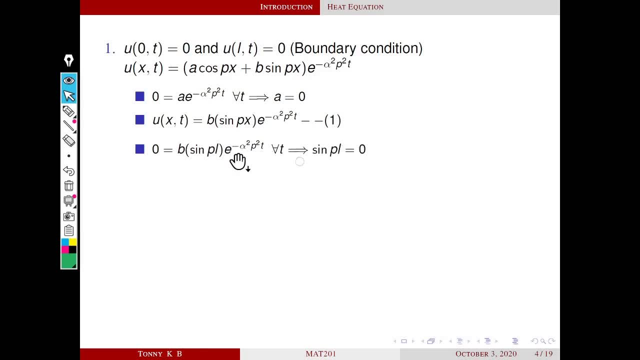 for every t and we know that this implies sin pl equal to 0. if b equal to 0, then solution becomes 0. similarly, if this term is throughout, 0 means solution becomes 0, so only possibility is sin pl equal to 0. sin pl equal to 0 implies what pl equal to n pi, so p equal to n pi by l and this: 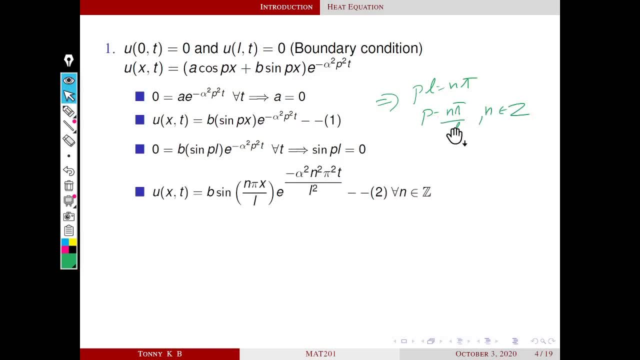 is true for every integer. we are substituting p equal to n, pi by l in equation number 1, then solution become u x, t equal to b into sin n, pi, x by l e raised to minus alpha square, n square, pi square by l square into t. this is our equation number 2 and this is true for every integer n. 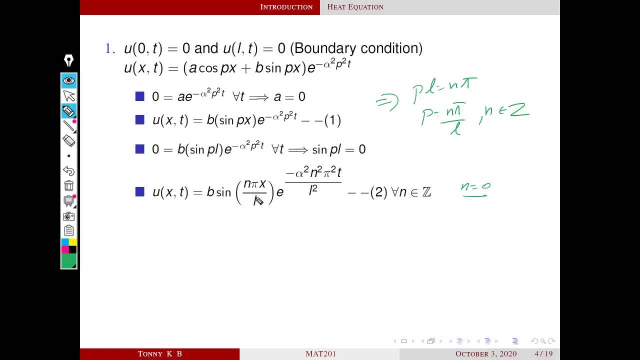 okay. if n equal to 0, this term becomes sin 0. right. when n equal to 0, this time becomes sin 0. sin 0 is 0. that means our solution is 0. we are interested only on um non-zero solution. we just remove the case n equal to zero. also, this is a solution for every n, so we 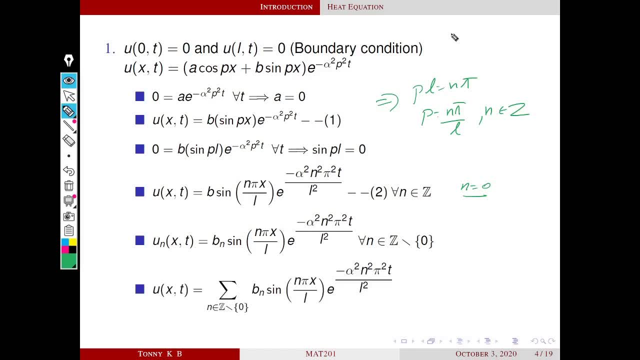 denote the solution by un of xt. also, we know that our integration is linear, homogeneous. okay. so if u1 and u2 are solutions of linear homogeneous, then there are some also solution. okay. so here all the uns are solutions of integration which is linear and homogeneous, so their summation is also: 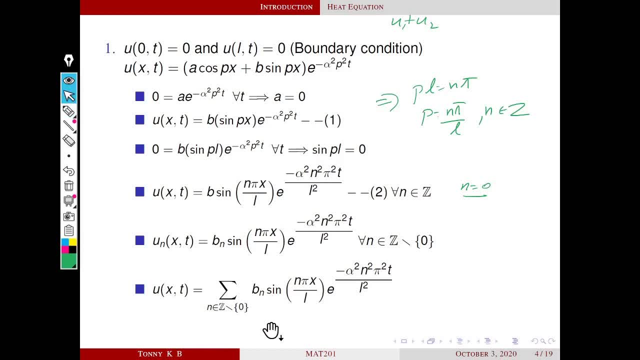 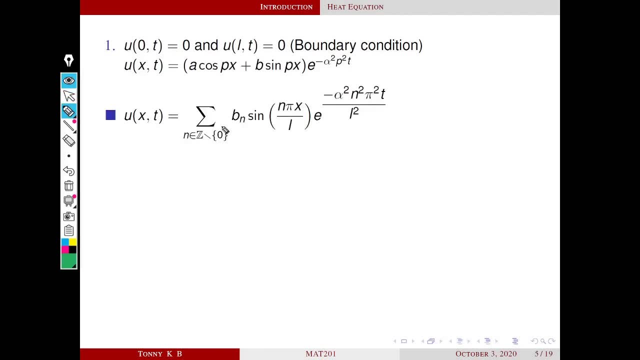 a solution: uxt equal to sigma n belongs to z minus zero bn sine n. pi x by l e raised to minus alpha square n, square pi square t by l square. okay, now the solution is like this: suppose n equal to, and what is the term corresponding? n equal to 2, that is b2. 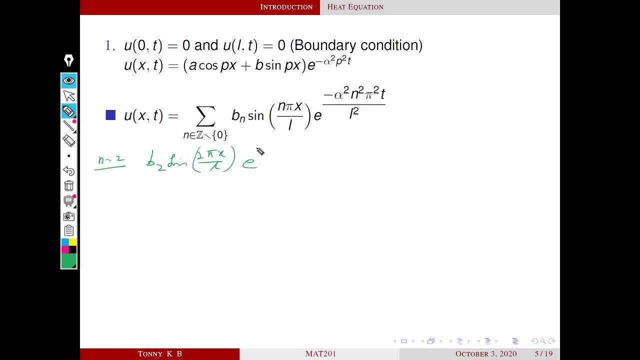 similarly for n equal to minus 2. what happened? b2? b2- the term is corresponding term- is b minus 2. here it is n square. so minus 2 square is again same 4. and we know that sine minus theta is minus sine theta. so this become: 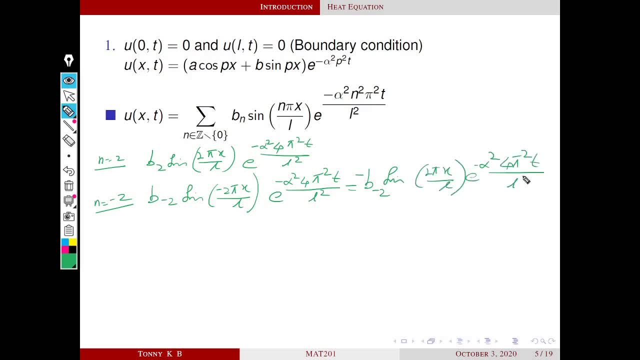 so this term is corresponding to n equal to 2 and this term is corresponding n equal to minus 2. it is clear that the terms are similar except the coefficient. you can compare the terms corresponding to n equal to 2 and n equal to minus 2. so what is? 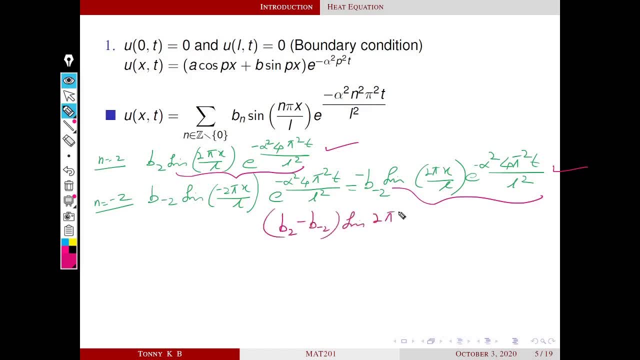 the resultant. the resultant is okay here. b2 and b minus 2 are arbitrary, so their difference is also another arbitrary number. so we can replace this arbitrary by some capital, b2, okay. similarly, you can compare the terms corresponding to 1 and minus 1 and 3 and minus 3, like that, okay, so 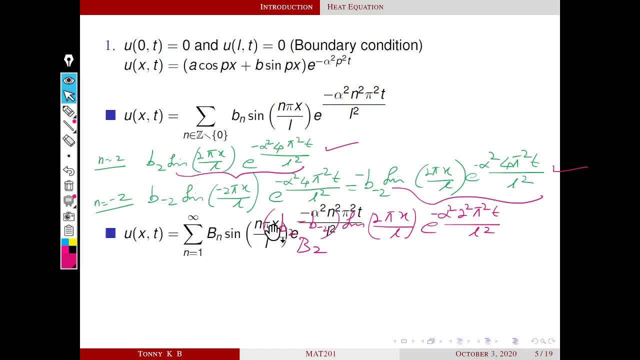 okay. similarly, you can compare the terms corresponding to 1 and minus 1 and 3 and minus 3, like that. okay, so our, our, our, these infinite series become uxt equal to summation, n equal to 1, to infinity, vn, sin n, pi, x, by l, e raised to minus alpha square. 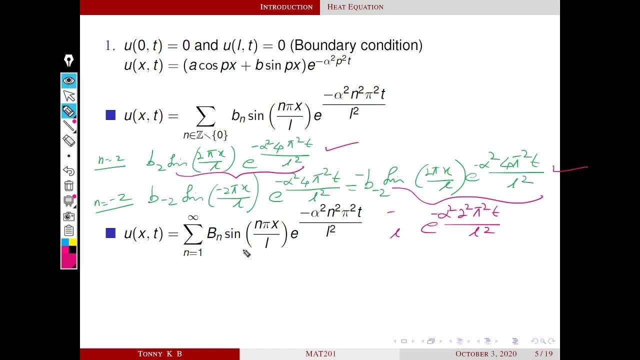 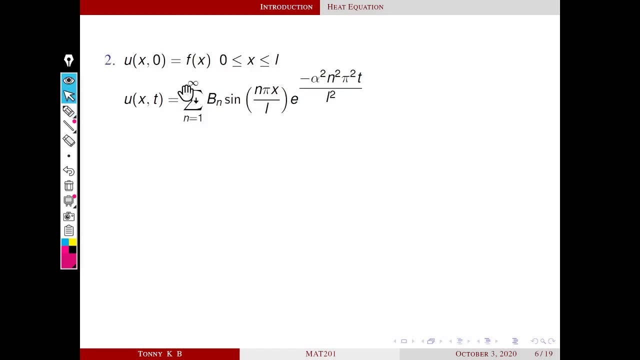 n square, pi square, t by l square. so next we have to find the unknown number's, vn's. okay, using our initial condition. okay, next we are going to apply our initial condition, that is, initial temperature, to our present solution. okay, when t equal to 0, our temperature is f of x. so you simply substitute t equal to 0 on the solution. 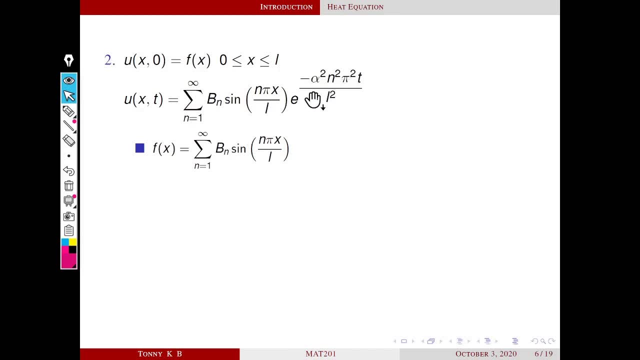 so left side will become f of x and right side will become when t equal to 0. this is e raise 0. we know that e raise 0 is always 1. what are we the n? this is always 1, so f of x is equal to sigma. 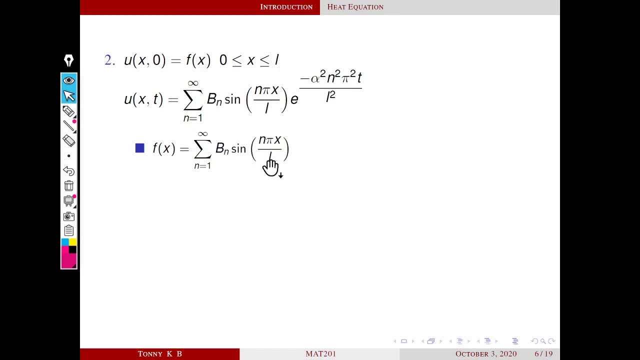 n equal to 1 to infinity. bn sine n, pi x by n. we know that. what is this series? this is exactly our Fourier sine series of f of x. so how to find bns? so bns are the Fourier coefficients. that is equal to 2 by l integral, 0 to l f of x sine n, pi x by l dx. so these two solutions are consistent with. 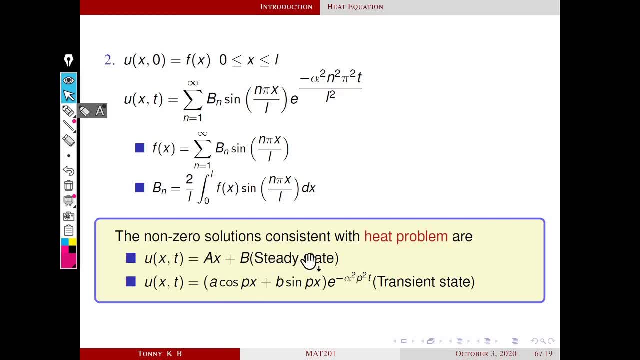 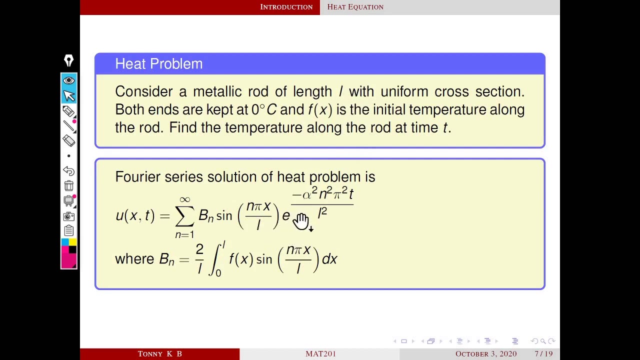 our heat problem and first one is our steady state problem. this is actually our third solution. the solution, the separable solution corresponding to k is negative. that solution is called transient state solution. so, as a conclusion, this is our heat problem and this is the corresponding Fourier series solution. okay, consider a problem: the ends of a homogeneous metallic rod of length. 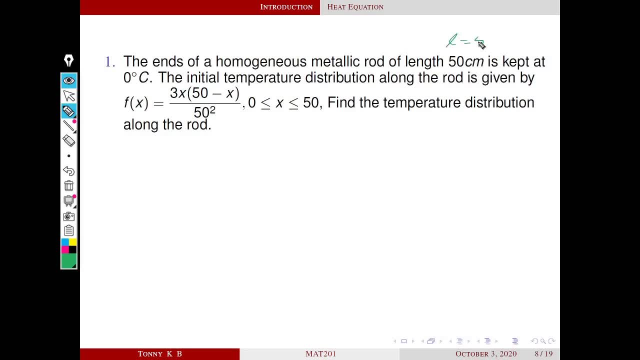 50 centimeter. so here l equal to 50 is kept at zero degrees. initial temperature distribution along the rod is given by: f of x is equal to 3x into 50 minus x by 50 square. find the temperature distribution along the row here. the given conditions are: u0, t equal to 0, u, 50 t equal to 0. 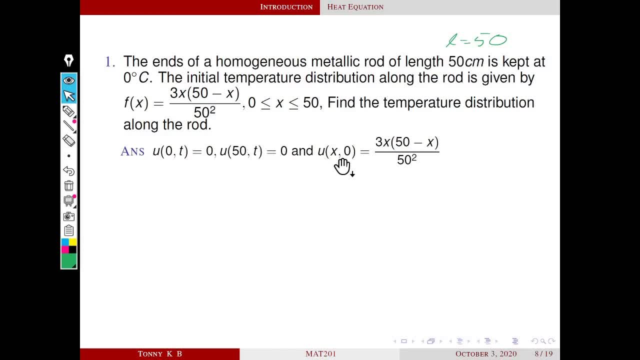 to 0 because l equal to 50 and initial temperature distribution that is ux 0, that is 3x into 50 minus x by 50 square. we know that this is our Fourier series solution of heat problem where bn is equal to 2 by l 0 to l, f of x into sine n, pi, x by l, dx. okay, we just replacing l by 50 and f of x by 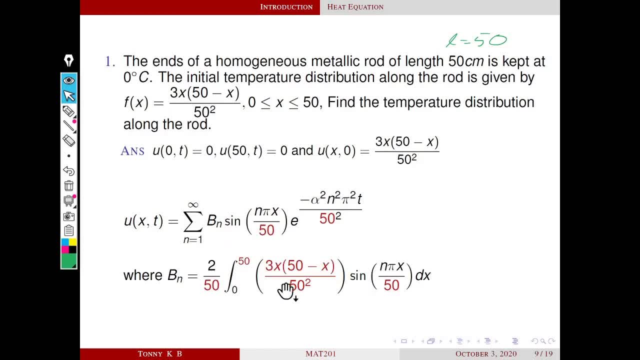 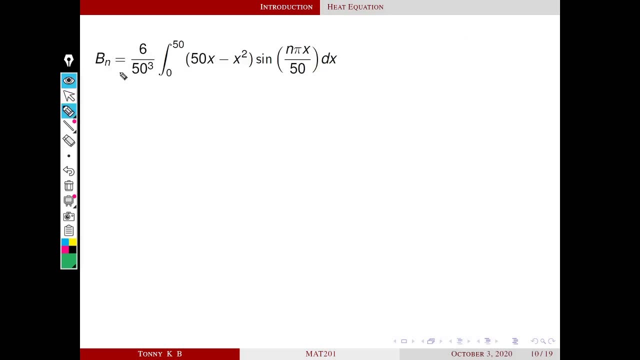 initial temperature. then we get like this: okay, so next we have to find bn by integrating this quantity. so here 3 by 50 square is common. you can take out, say so, this becomes 6 by 50 raised to 3.. so bn is equal to 6 by 50 raised to 3, integral 0 to 50. 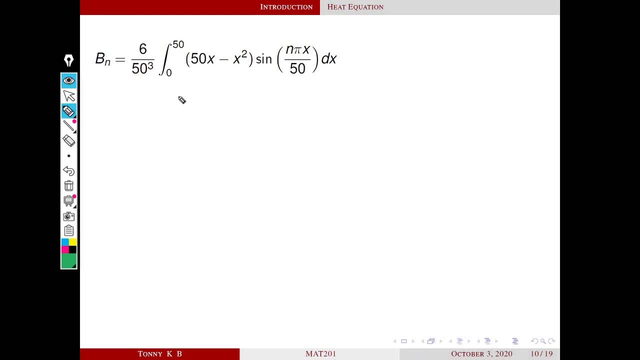 50 x minus x square into sine and pi x by 50 dx, then we use integration by parts, the general rule of integration, that is nothing integral. uv dx is equal to u into v1 minus u1, into v2 plus u2, v3 minus plus, etc. here lower suffixes for integration, upper suffixes. 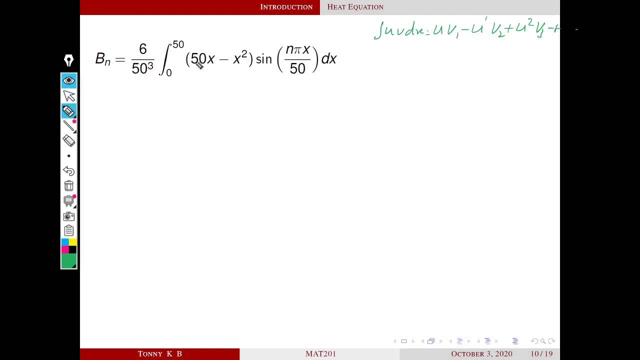 for derivative. okay, by applying this rule, this integration become like this: first function. this is our u, this is our v1. v1 means integration of this v. okay, that is like this: minus cos n pi, x by 50, n pi by 50 and minus u dash. u dash means derivative of u, that is 50 minus 2x, into v2. this is our v2. what? 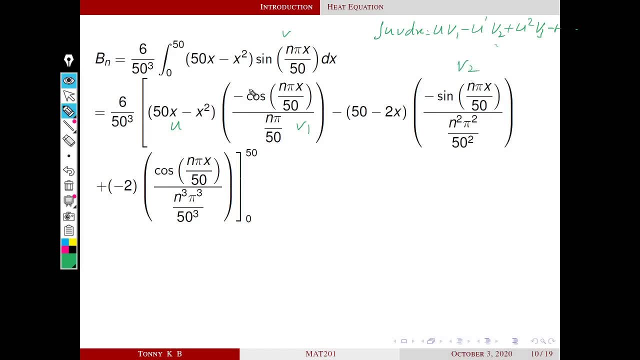 is v2. v2 means integral of v1. v1 is entire thing. okay, this entire thing is v1. so that is minus sin n pi x by 50 divided by n square, pi square by 50 square. then plus u2. u2 means derivative of u1. so 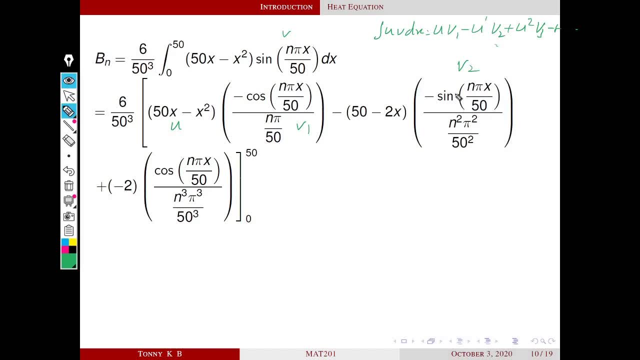 its derivative is minus 2 times integral of v2, that is v3. so v3 is cos n, pi x by 50 by n q, pi q by 50 q. okay, the limits are 0 to 50.. when x equal to 50, this term is 0, 50 square. 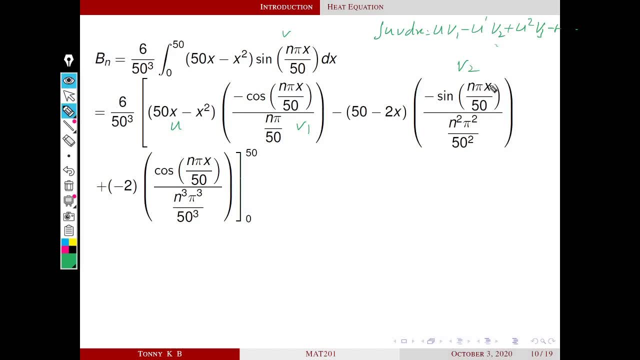 minus 50 square is 0 and this term is x equal to 50. this is sine and pi right sine and pi is 0 and this term become cos n pi. so this expression become 6 by 50 cube into 0 plus 0. this become minus 2 times. you take the reciprocal of this one, so 50 q by n cube, pi, cube. 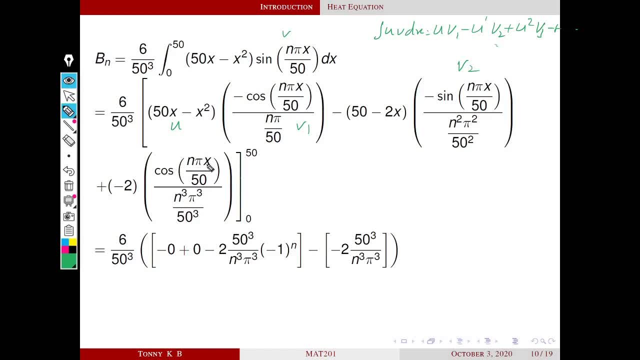 into this is cos n pi when x equal to 50.. so cos n pi is minus 1 raised to n minus. next we substitute the lower limit when x equal to 0. this term is 0 when x equal to 0. sine 0 is 0 when x equal to 0. 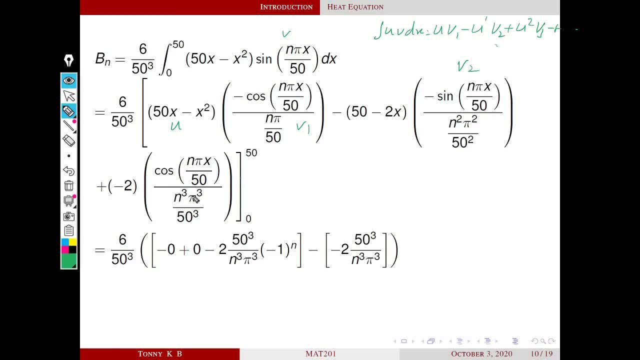 this is 1 throughout 1.. so minus 2 times its reciprocal, that is 50 q by n q pi q into, this is 1. here 50 cube is common in numerator. you can take outside and cancel. then 2 by n q pi qb is also common. okay, so upon simplification this become 12 by n q pi cube into. 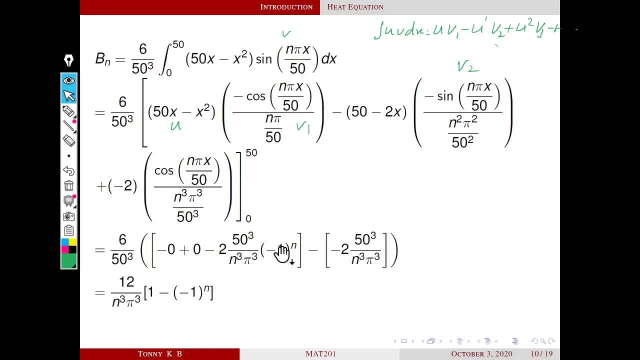 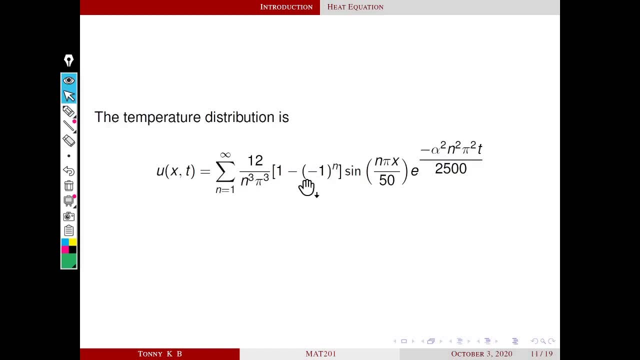 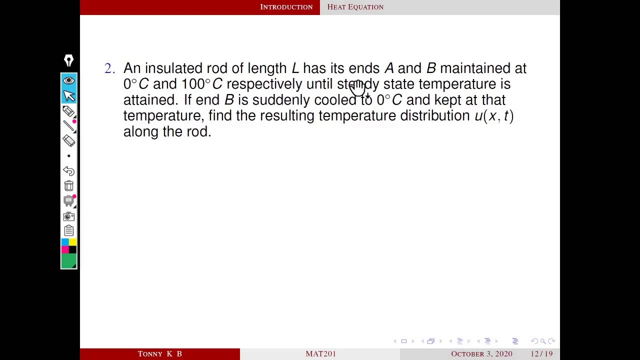 this term is 1, so 1 minus. this is minus of minus 1 raised to n. so this is our bn. so by substituting bn in our uxt. so this is the final temperature distribution. next problem: and insert road of length l here as its ends a and b, maintained at 0 degree and 100 degree. 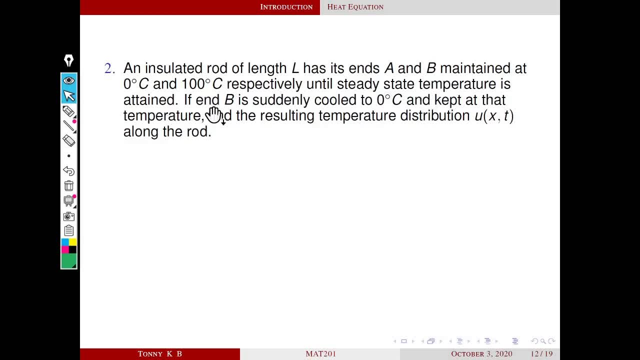 respectively until steady state temperature is attained. if end b is suddenly cold to 0 degree and kept at that temperature, find the resulting temperature distribution uxt along the road here: 0 degree, 100 degree. okay, this is our t1, this is our t2. then what is the steady state when one side is? 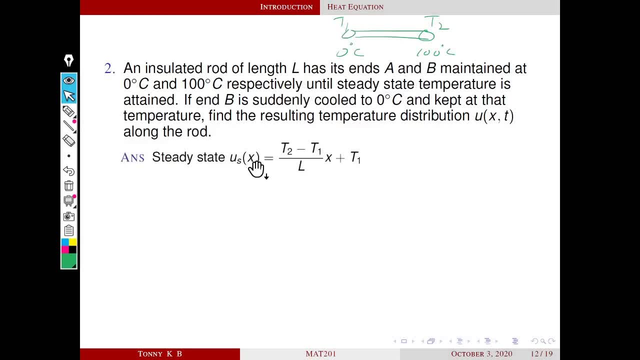 0 degree is 0 and the other side is 1 plus t1 and other side is t2. this is the steady state temperature. usx is equal to t2 minus t1 by l into x plus t1. so here t 2 is 100 and t 1 name is 0. 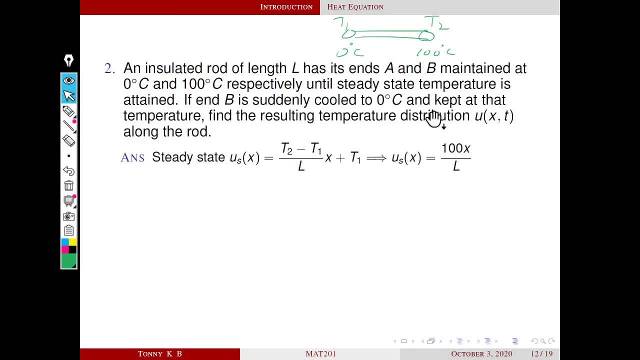 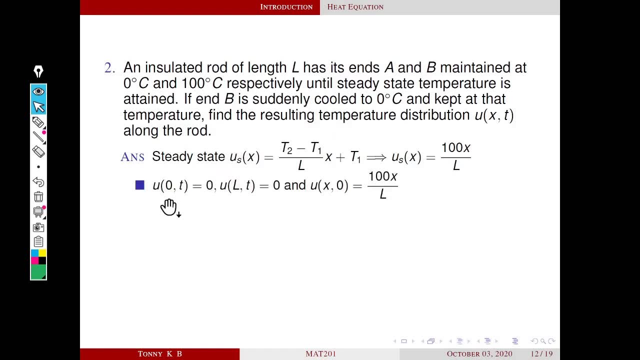 so this will become hundred x by n. so this is our initial temperature distribution. then we suddenly change the temperature h b to 0. so our solution, UXT, should satisfy: U zero, t equal to 0, and u t is 100 phenomenal l t equal to 0 and u x- 0 equal to 100 x, 100 x by l. so this is our Fourier series solution. 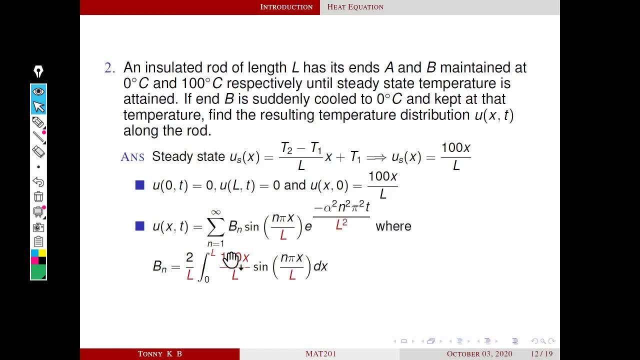 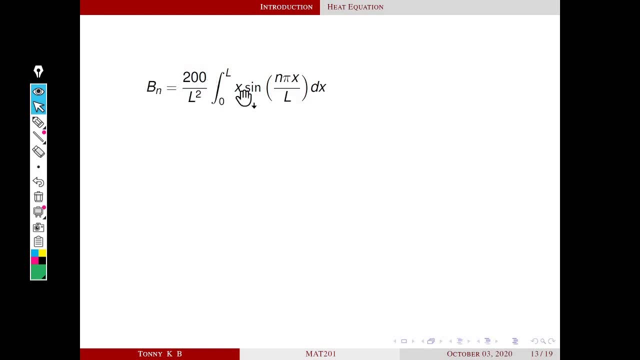 and where b n is equal to, like this: 100 by l is constant, so you can take outside, so this become 200 by l square, so b n is equal to 200 by l square, into integral 0, to l x, into sine, n, pi, x by l dx. then by integration by parts, this become x into first function, into integral of. 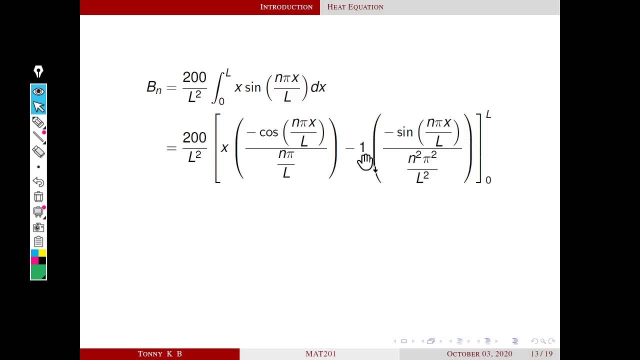 second, minus, derivative of first, that is 1, into integral of this, this term, that is minus sine n pi, x by l divided by n square by square by l square, and limits are 0 to l and x equal to l, this become l into minus, cos n pi by n pi, by l, n pi by l become l by n pi. so this term is 200 by l square.